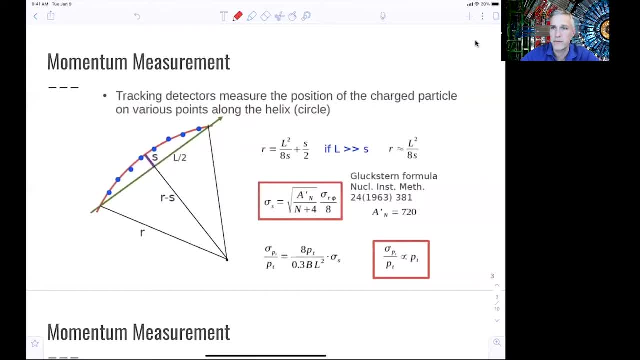 trajectory. So this is typically done with tracking detectors, And so what you then measure is not the radius directly, but you measure individual points as part of the trajectory of the particles, And so from the measurement of the points you can then reconstruct the trajectory of the particles. 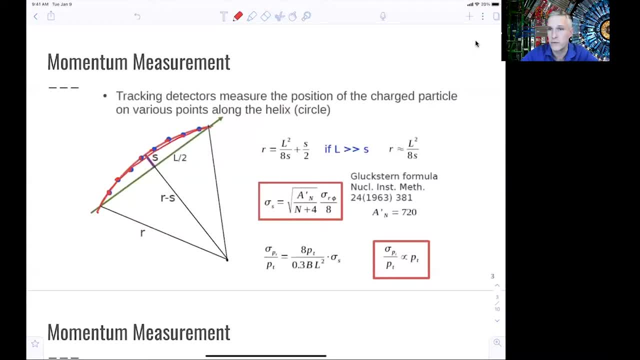 and then therefore measure the curvature, And that has been used to measure to the transverse momentum. So if you look at this picture, here the radius can be given as l square over 8s plus s half. s is typically called the sagitta of the trajectory. 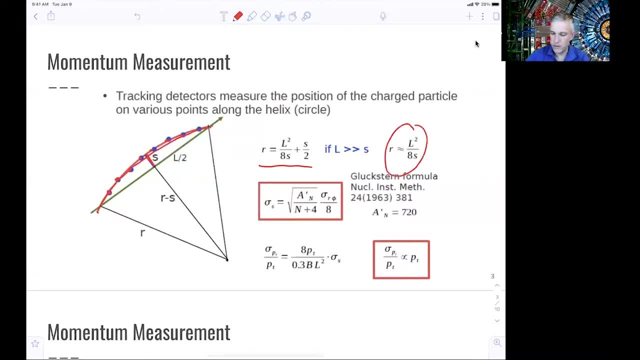 If l is much, much larger than s, it simplifies to about l square over 8s And the uncertainty on the sagitta, the uncertainty on s, is limiting the uncertainty on the momentum, And this is described in a paper which is very nice, from the 60s. 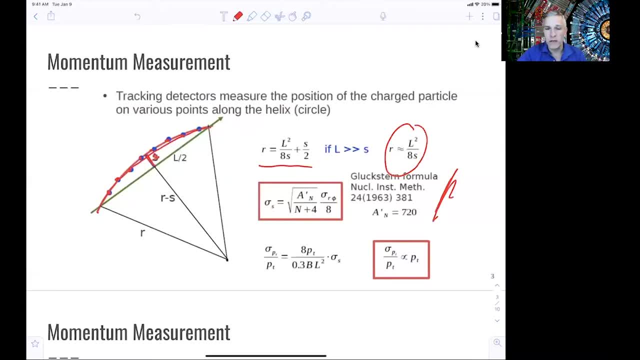 And the formula is called the Klug-Stamm formula. So what you see here is that the more measurements you actually perform along the sagitta, the better your measurement is performed, And this goes with a square root of 1 over the number of measurements. 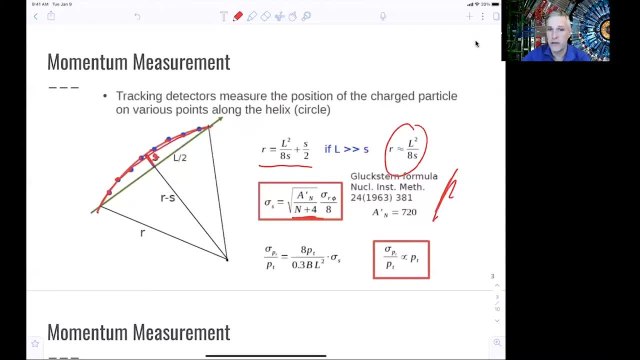 The total momentum uncertainty or the relative momentum uncertainty sigma pt over pt is proportional to the uncertainty- uncertainty on the circuit- And that also is then proportional to the PT of the measurement. So if you want to improve your measurement of your momentum, 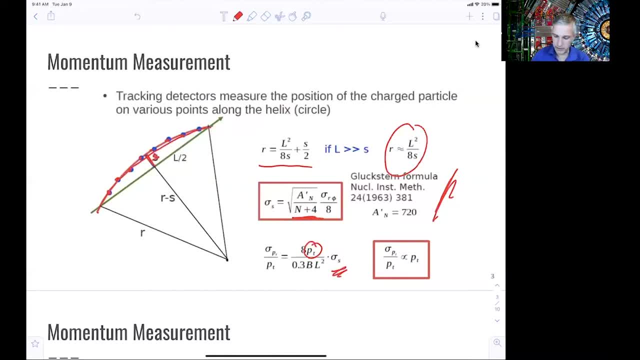 you want to decrease the uncertainty And you can do this by having a large L And you see, this goes with the square of the length. You want to increase your magnetic field And you want to reduce the uncertainty on the circuit. Those are the elements you have in play. 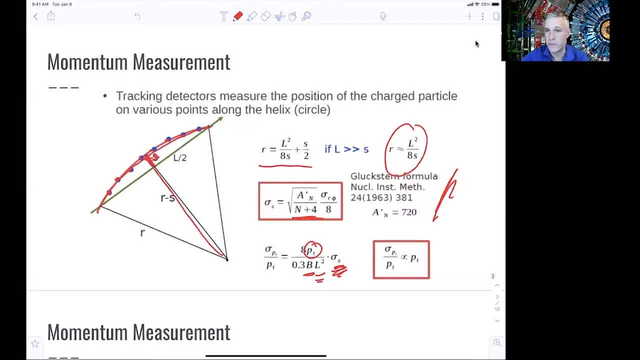 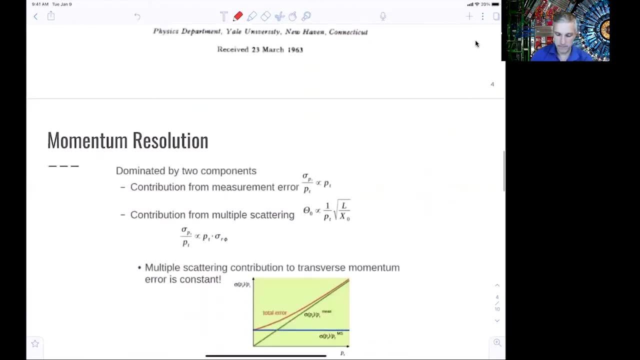 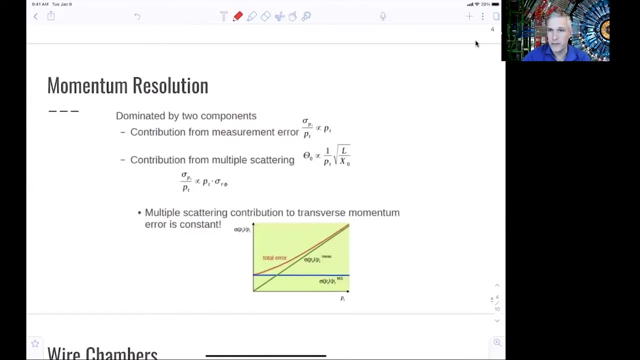 in order to improve the transverse momentum or the momentum measurement of your charged particles. So this is a screenshot of this paper. The measurement error is not the only error on the transverse momentum, as we discussed previously already, Multiple scattering, So the scattering. 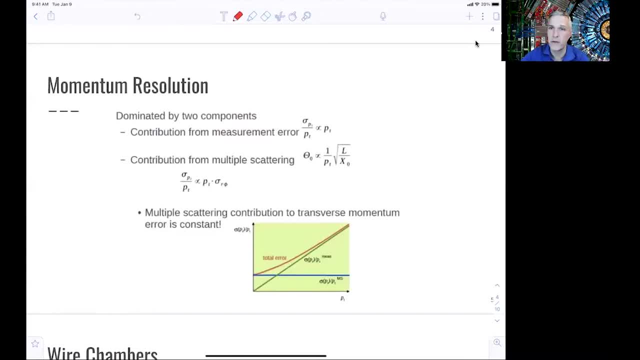 The scattering of the particle as it goes to the momentum also reduces the uncertainty on the momentum measurement And we can show that this component on the relative momentum uncertainty is flat. So what you find typically is that the transverse momentum measurement is limited at high PT through the measurement error. 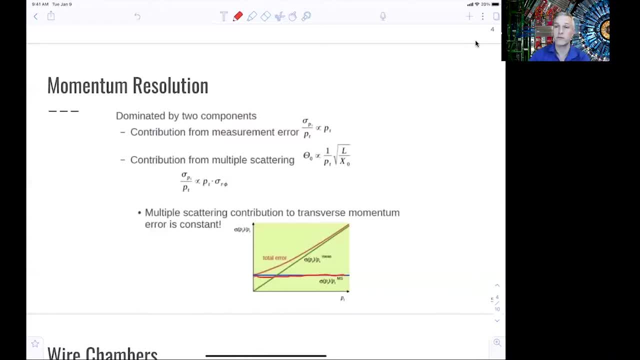 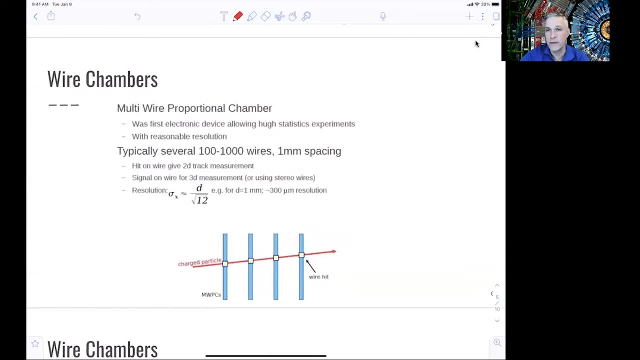 and at low PT through multiple scattering. So you have those two components entering the measurement uncertainty. So the actual detectors. I just give you a couple of examples here, The first one and the first one which actually really has allowed to make measurements with a lot of devices. 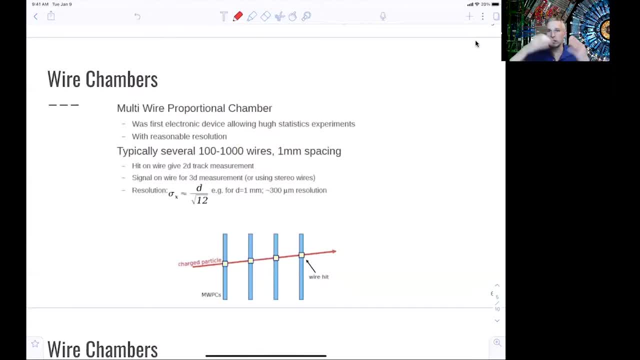 with huge statistic experiments where you have been colliding beams and you look at many, many of those interactions. was the multi-wire proportional chamber At a reasonable resolution? typically we have hundreds or thousands of wires with a spacing of up to one millimeter. 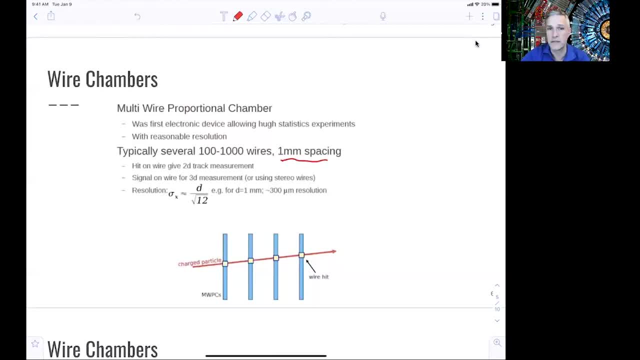 And this one millimeter spacing in the wire chamber limits the spatial resolution. If you don't have any knowledge of where the particle was in the flat area, then the uncertainty of the spatial on this one hit. uncertainty is given by d, the spacing between those two wires. 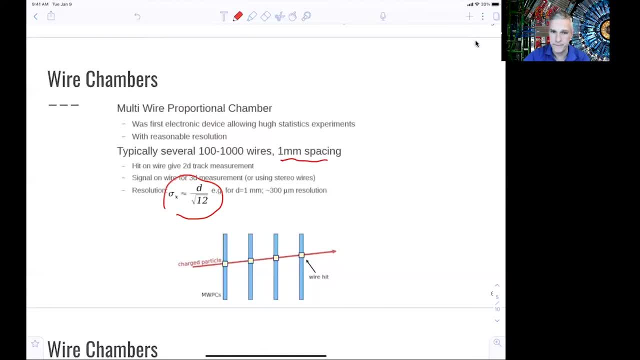 one millimeter, in this case, divided by square root of 12.. So you find typical resolutions of 300 microns per measurements, but you make gain of the fact that you typically have many, many, many measurements And, as we just saw, this reduces uncertainty. on the measurements. 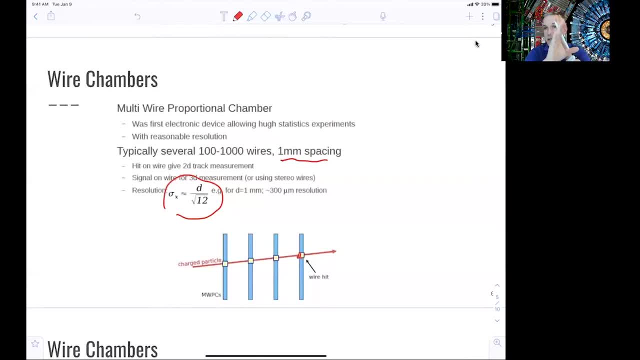 If you then build the wire chamber such that there's angles between individual wires, you can use that in order to gain three-dimensional information from the geometry of where the 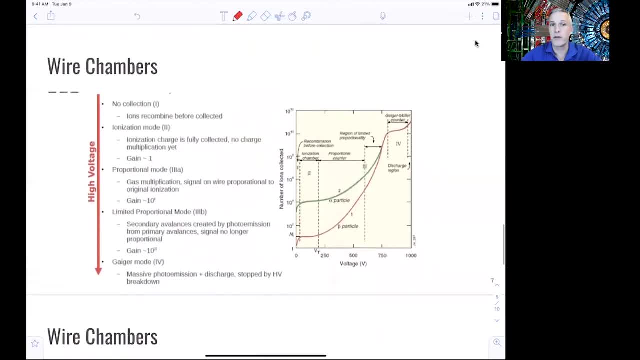 particle went through. Wire chambers can be operated in different modes and it depends on the level voltage you apply on the wires. So the higher the voltage, the level of the voltage goes down here. If you have very limited voltage applied, then you have ionization and the ions recombine without. 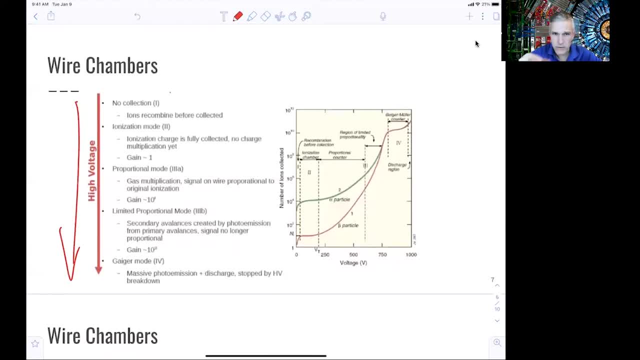 being collected In ionization mode. you collect the ions and there's typically a gain factor of one. You measure each ion basically separately. You can increase the voltage and run the wire chamber in proportional mode, So you have a gas multiplication factor. So the ions are being 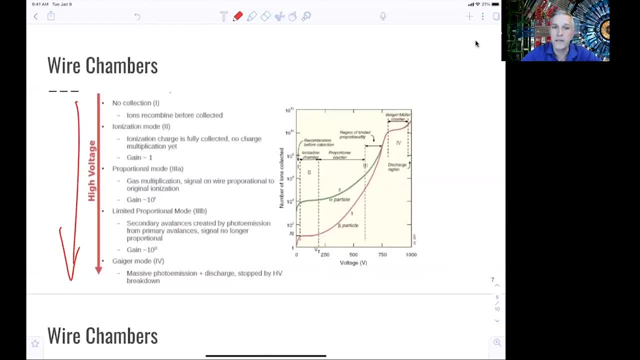 accelerated, and then they produce many more ions to be measured, And you typically have gain factors of 10 to the fourth. If you drive this further up, you go into the limited proportional mode, And then it's Geiger mode, where you basically have an avalanche, And so you have no information. 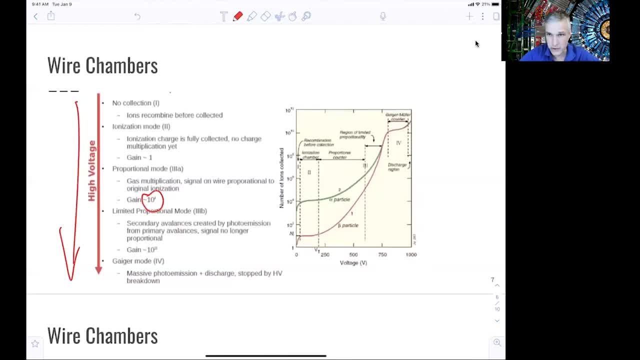 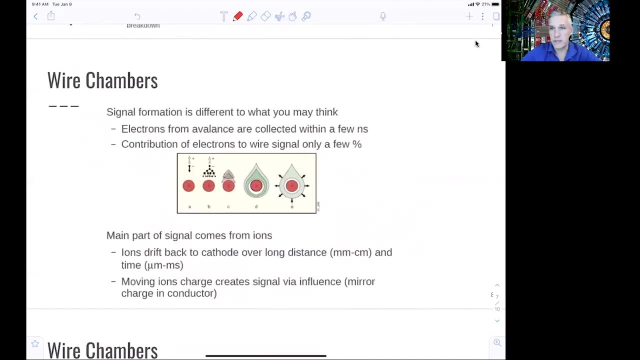 about the initial ionization anymore, And typically the chamber breaks down and needs to recover afterwards. The signal formation is quite an interesting concept. So you think that you do ionization. the electrons are there and then they're being collected. Yes, that's true And this happens. 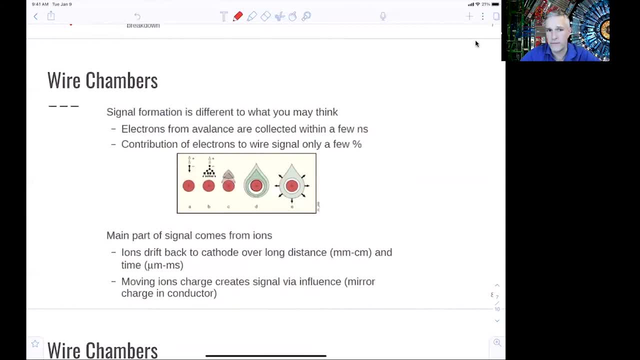 very rapidly, typically in the order of nanoseconds, But the actual, real signal comes from the ions themselves, And so what happens here is: you have your wire here, You have your electrons, The ions, then themselves they build this cloud of charges And this cloud. 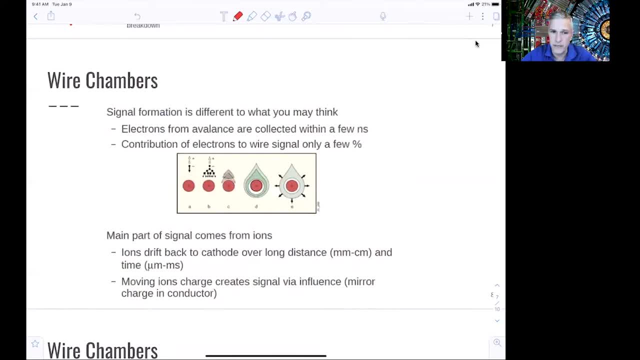 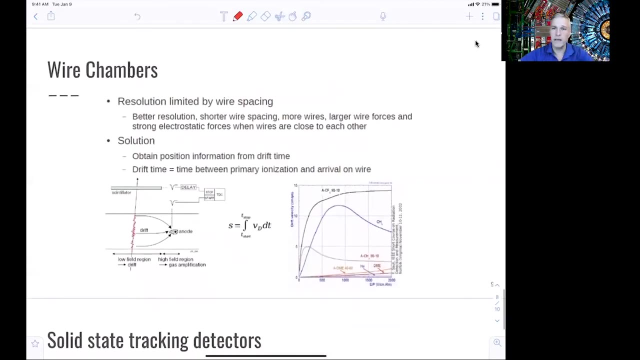 of charges then gives you a signal on the wire, And this happens typically via influence, or you basically have a mirror charge on the conductor, And that is really where the bulk of the information comes from. We just discussed that the spatial resolution is limited by the spacing of the wires. 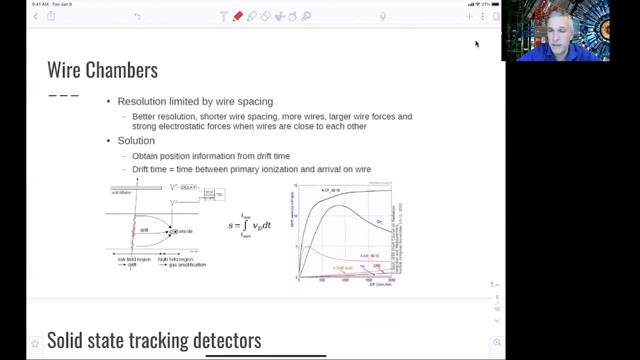 You can actually get better measurements by using the timing information. If you are able to measure the time profile of your signal, that profile has information about the distance between the ionization and the wire itself, And that then helps you to improve the resolution further. 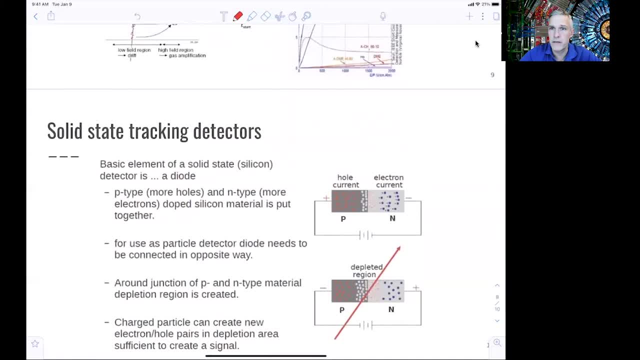 So I really don't do justice to this, But nowadays, specifically in high-dense, particle-dense environments, we use solid-state tracking detectors And they're used in many, many, many areas. in particle physics, The idea is to use mostly silicon. 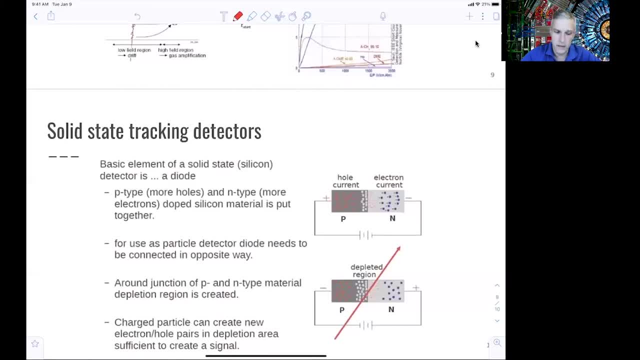 but you can use other semiconductors as well. You dope them, meaning that you create more holes by using p-doping and n-type doping for more electrons, And then you bring n-doped and p-doped materials together And it's the same way as in a diode.